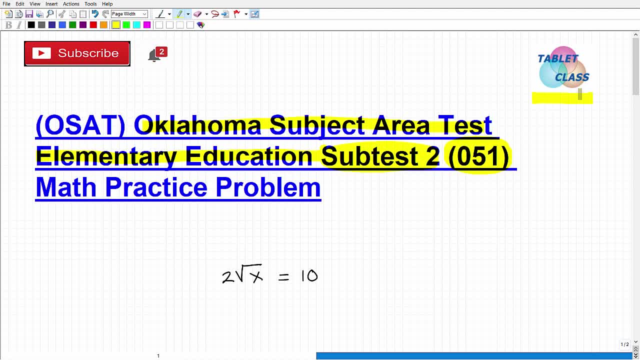 Let me go ahead and introduce myself. My name is John. I'm the founder of Tablet Class Math. I'm also a middle and high school math teacher And over several years I've constructed many online math courses, very comprehensive math courses to include an Oklahoma subject area test, elementary education subtest to 051 test prep course. I'm going to leave the link to that in the description of this video And the way I construct my test prep courses. I actually go in. 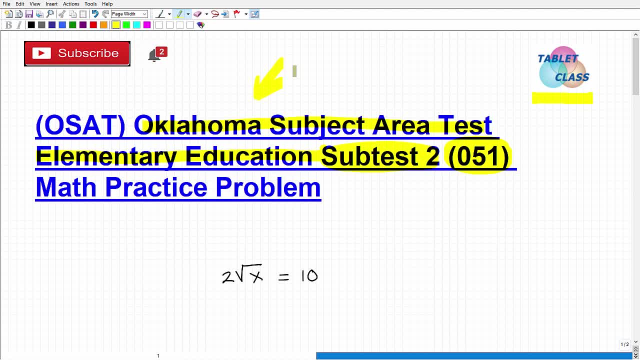 and research. you know the specifications are going to be on the test a particular type of math and try to create a very customized math course. So I don't want to give you too much math, I don't want to give you too less math, because there's other OSAT certification exams. all depends on what you're going to be teaching, whether you're gonna be teaching middle school or high school, etc. So the math requirement could can change dramatically. Okay so 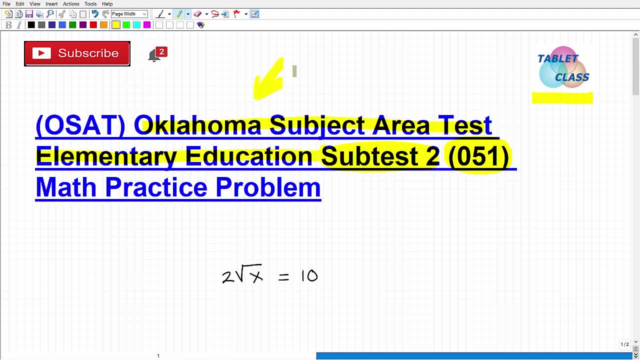 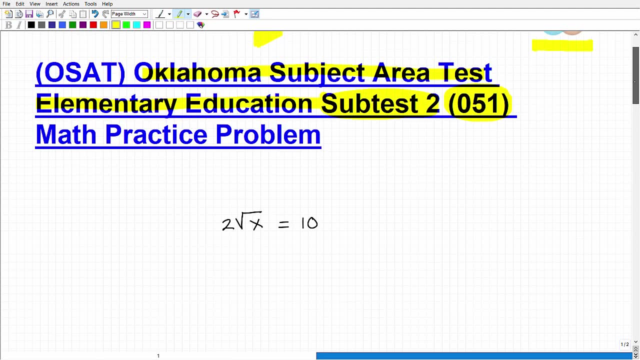 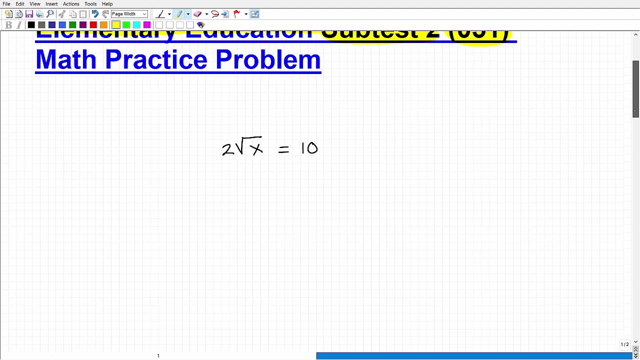 this particular test I would kind of classify: the math that you need to know is kind of high school level mathematics- maybe not super, super advanced, but you're definitely going to have to be strong in algebra and geometry and other topics as well. So a problem like we're going to take a look at here falls into basic high school kind of level math. So let's get into the problem And here we have an equation. So obviously I'm going to solve it. But the way I like to kind of do these 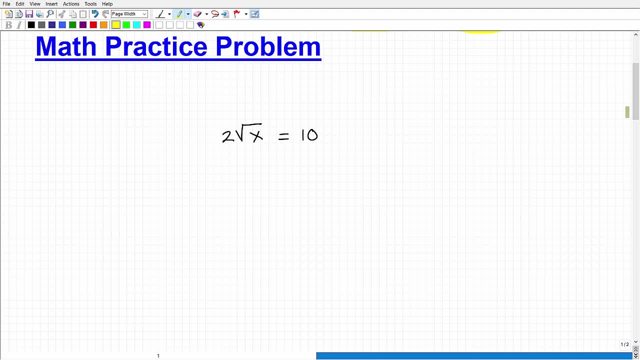 videos is give you an opportunity to pause the video. you know, think about it. you know you should try to do the problem on your own. don't go to Google, don't look up how to do it, just kind of go by memory, play around with it, even if you're not sure you know. think about if you were given this problem how might you kind of approach it. So that's the first kind of phase of this video. then I'm going to give you a little bit of a hint here in a second to kind of help you along. then obviously I'm going to 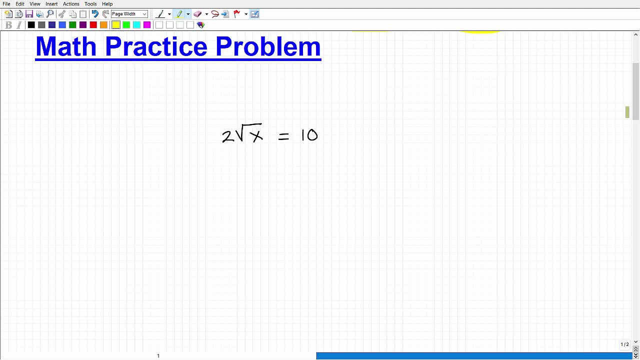 solve the problem, Okay. so if you don't want to hear the hint, go into, pause the video and try it. Try the problem. So now I'm going to give you a hint, All right? So here let's take a look. Obviously, we have an equation, right? So let's take a look at a more basic example. So let's get rid of that square root. So if I had two, x is equal to 10, hopefully you will know that. okay, I have to divide both sides of the equation by two, So x would be equal to five. 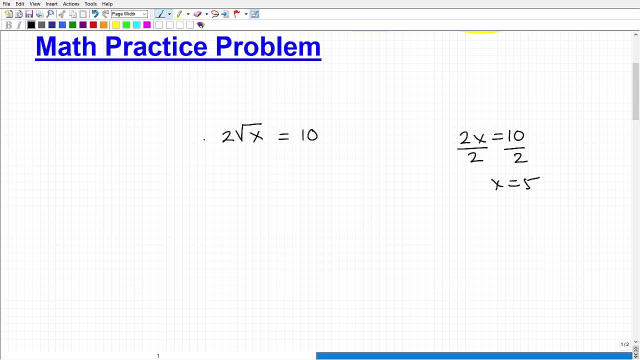 Okay, so same thing here with this particular equation. what you want to do you're not solving for x. what you're going to be doing is trying to isolate the square root or the radical. Okay, so you're going to be left with just radical: x equals some number. So when you're dealing with radical or square root equations- this is the first kind of phase of the problem- Okay, so, basically, isolate the radical. So now, when you isolate that radical, 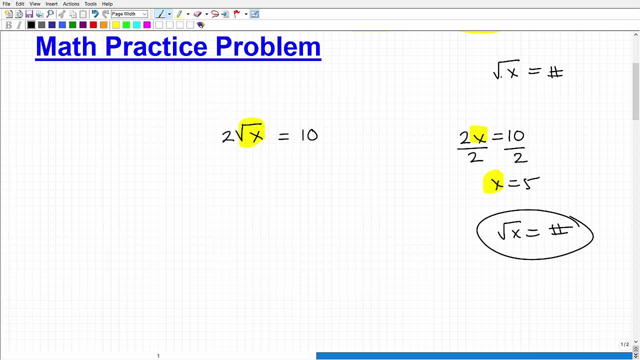 how do you solve this problem? Okay, so I want you to think about that. I'm going to obviously show here in a second- And this is just a basic example- these type of problems. But let's just take a look at this equation: square root of x equals four. Okay, so let's just kind of discuss this, what this means algebraically. the square root of x- Now remember, x is a variable in an algebra, variables just basically represents a number. 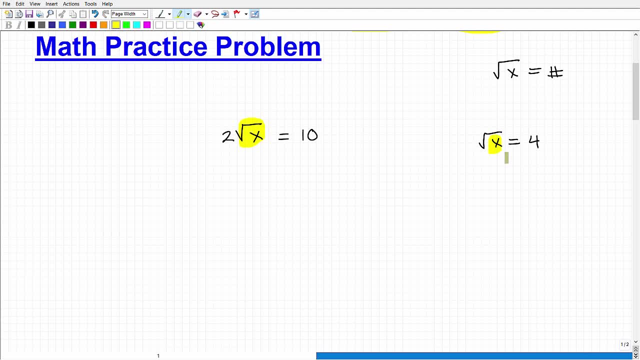 Okay. so what if I just came up to you and I said: Hey, excuse me, the square root of what number is four? Okay, do you know what that is? What is my my calculator is telling me? for I took the square root of some number and our answer was four. Okay, hopefully you'd be like, Oh yeah, if you take the square root of 16, the answer is four. it's technically positive, negative four, but you kind of get my drift here, right? So you know, looking at this, 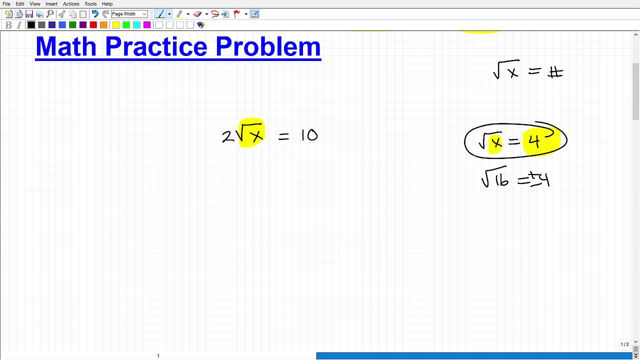 you can kind of, you know, just deduce what the answer may be. But there's a little bit more of a formal way. we want to go ahead and approach radical equations, And these little things here are called radicals or square roots. So, with that being said, let me go ahead and solve this real basic problem, And then we'll wrap up this video, So okay. so again, first thing you want to do is to isolate the square root of x part, So I'm going to divide both sides of the equation by two. 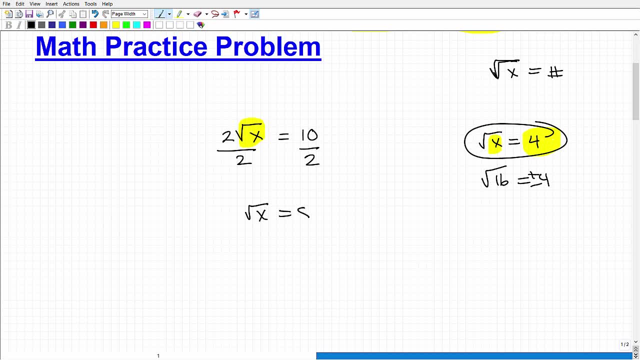 So I get: the square root of x is equal to five. So again I could say: the square root of what number is five. So hopefully you know the answer is 25, right? Oh, the square root of 25 is five. Again, the square root of 25, when you're taking the square root of a real number, you have two answers. you have a positive and negative five, because positive five times positive five is positive 25 and negative five times negative five. 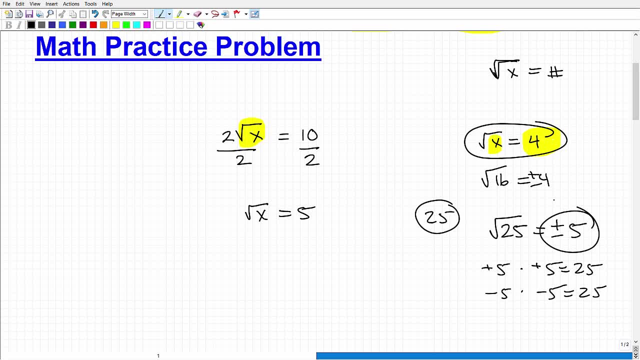 It's also a positive 25.. So this is the real, the most like, technical, most accurate, complete answer. But you know just to kind of. you know I don't want to get too deep into this topic because there's other things that come up when you're talking about square root equations or radical equations, but just want to kind of keep it basic here. But I just I wanted to again just to reiterate: when you're taking the square root of real number, there are two solutions like this: 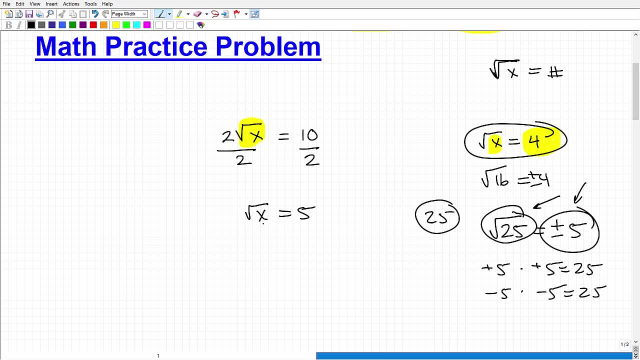 All right, but let's get back to our problem. So I have: the square root of x is equal to five. Now, in this case it's pretty easy, because you're thinking: oh, the square root of some number is five, Oh, that's 25.. But what you really are doing mathematically is: you want to, you want to get to x. right, we want to solve for x, but I have a square root here. So the way to get rid of that square root is to square a square root. So if I square this square root of x, I'm left with x, But if I square the square root of x, I'm left with x. 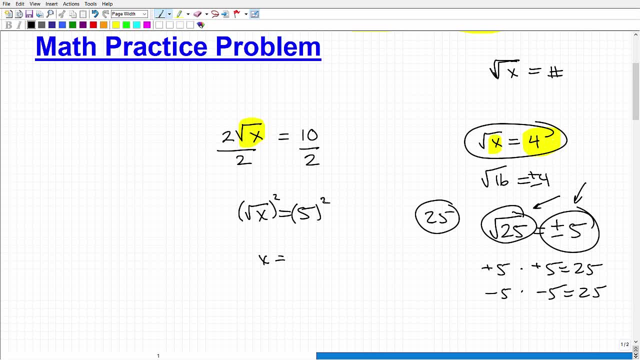 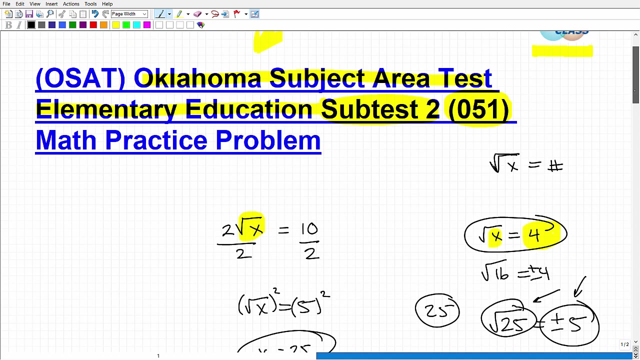 But the left hand side. I also got a square of the right hand side. So five squared is five times five is 25.. And that is our solution. So anyways, again, this is a real basic example or basic level square root equation. okay, something definitely you should be able to handle if you're fully prepared for the subtest to on this particular Oklahoma subject area test. 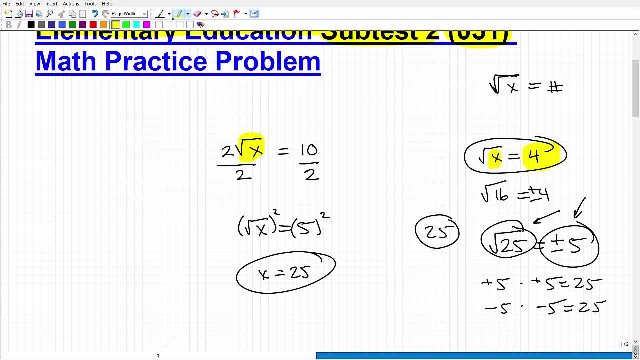 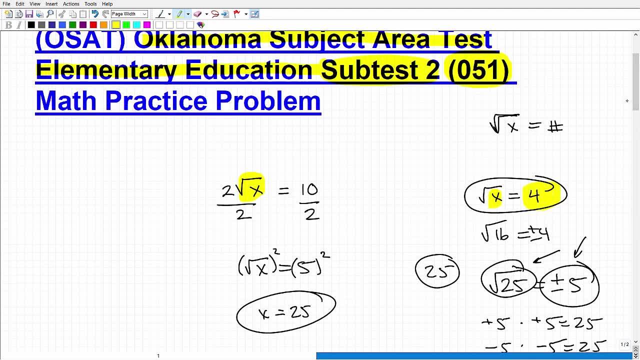 Yeah, Now, if you got this right, that's excellent. Okay, if you didn't need a hint and you understood what you were doing, that's fantastic. But by no means is that complete verification or validation that you're ready for everything. that's on this test. Okay, there's a lot of other material that is on all the math topics. on the math topic is on here. Now, if you didn't get this right, if you struggle with it, don't panic. just use it as feedback to get serious about you know studying, So let's go ahead and wrap up this video. I'm 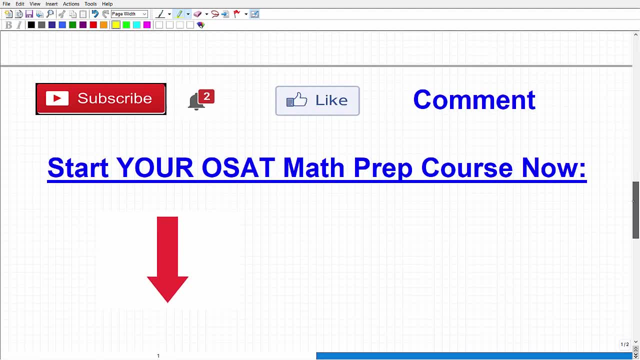 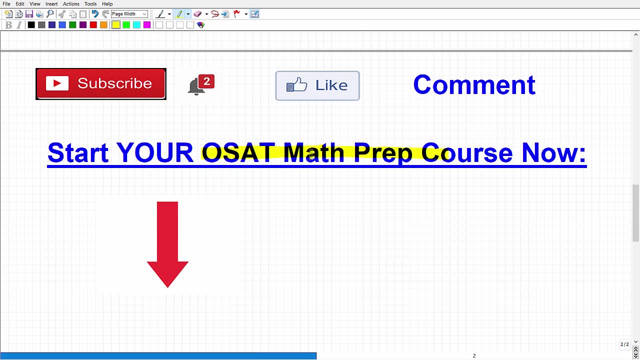 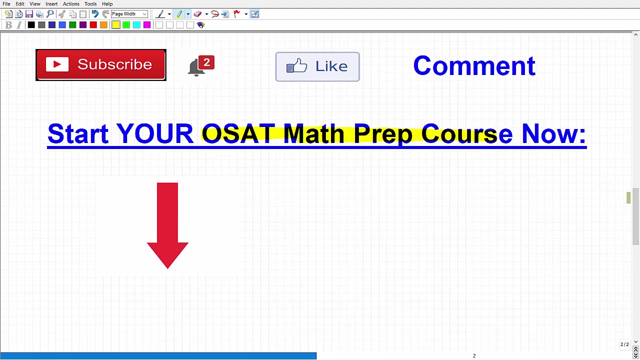 going to go ahead and stress some things I like to do In all these videos. again, I'm going to go ahead and leave a link to this particular OSAT test is 051, my math prep course for it in the description of this video. you can check that out, But I'm going to leave you with these comments. If you're new to teaching- and you may or may not be new to teaching One- you want to take all certification exams very seriously. Okay, I'm sure you've 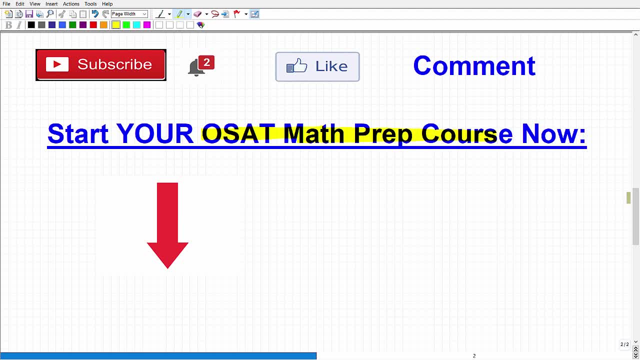 just by virtue of you watching this video. But what I mean by that is: don't underestimate any exam. Okay, And I think at the elementary level, especially with mathematics, a lot of elementary school teacher candidates or people who haven't taken these exams might kind of think that, well, you know, maybe I just need to know elementary level math. you know place value, decimals, fractions. of course you need to know all that, But you really need to take a look what's on the exams. And again, most of the times, 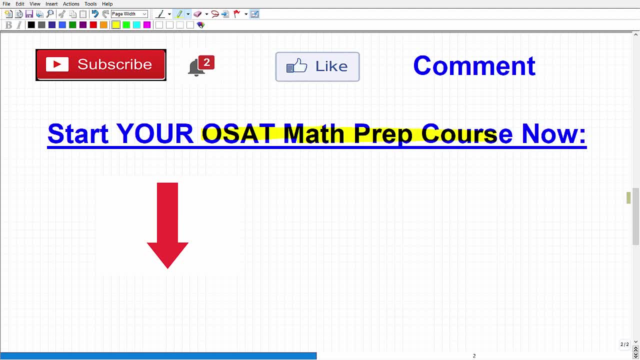 Most elementary level. certification exams throughout the United States, depending on what state you're in, are going to require you to know a good amount of high school level math. OK, so just because you're teaching elementary doesn't mean that you're going to escape algebra, geometry, etc. 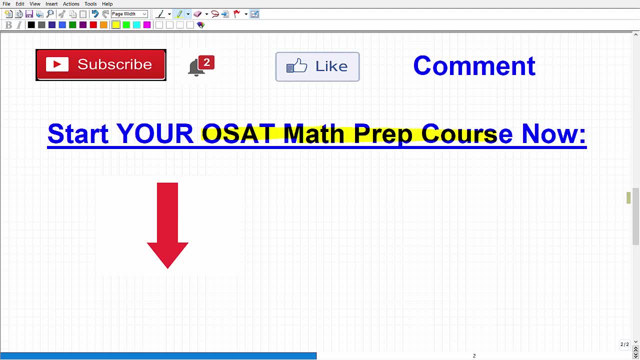 So do your due diligence and come up with a good study plan. Study hard so you don't have to take this exam once and move on. OK, you may or may not know this, but there are plenty of teachers out there that fail the first time out, have to go back a second time or a third time to actually pass exams. 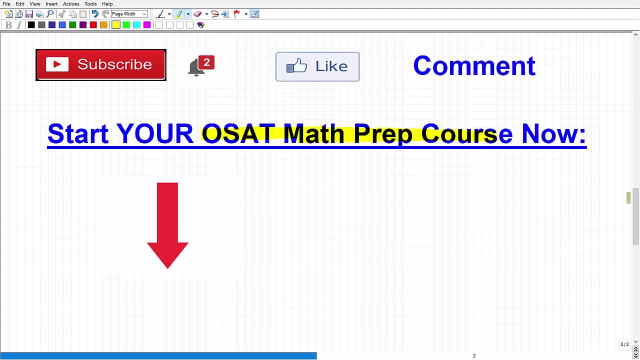 If you study correctly the first time out, you won't be one of those teachers. So anyways, you know. I'd just like to kind of stress that point. But if you're new to my channel, hopefully consider subscribing. I've been on YouTube several years. 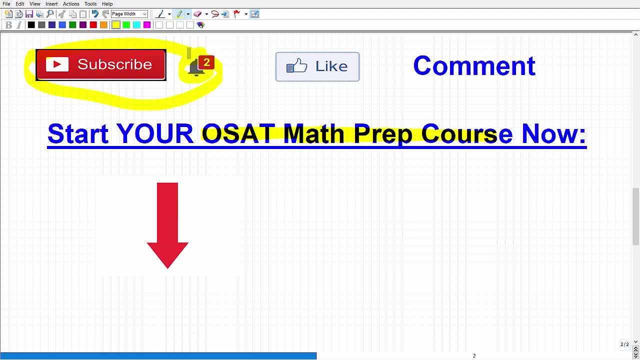 I already have all my channels, several hundred Videos that can help you prepare for this particular exam, So hopefully you'll check that out If you like the video. definitely, appreciate a thumbs up and leave me some feedback. Are you coming from a different level of teaching or maybe a different state? 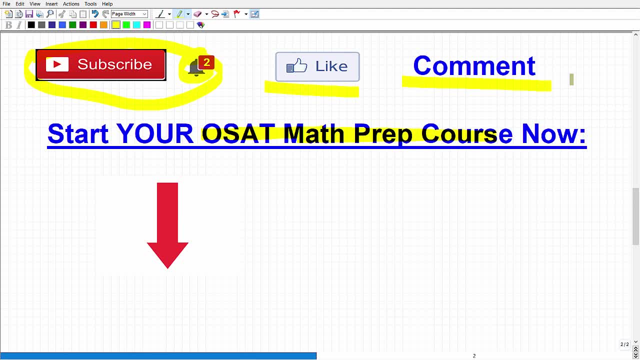 Are you new to teaching? Are you coming right out of college, right from high school to college to teaching? Or maybe you're doing a career transition, you know, coming from one career into teaching. So you know, these days there's a lot of different ways you can. 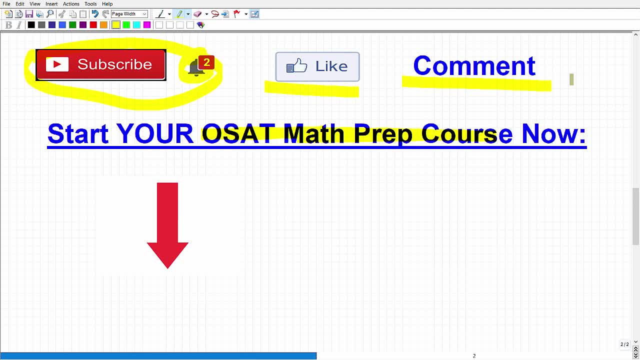 Be a teacher. I think that's actually a good thing because we need as many good teachers as possible And I always like to kind of throw in my little two cents to kind of show my- you know- support for fellow teachers. is that, you know, being a teacher is it's challenging work but it's also rewarding. 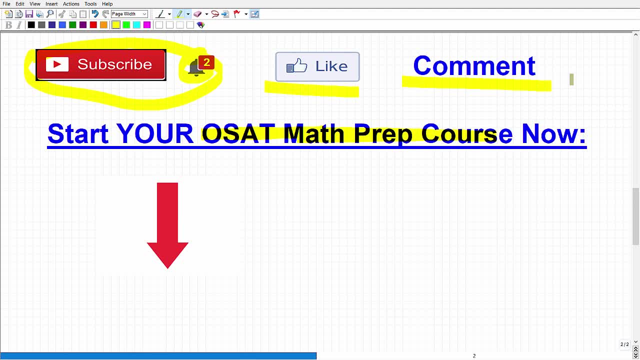 OK, unless you have actually been a classroom teacher. everybody thinks they know what it's like because they see a teacher in the classroom. Oh, I could do that, Oh, and you get summers off as well, and et cetera. But you know that's this kind of goes with the territory. 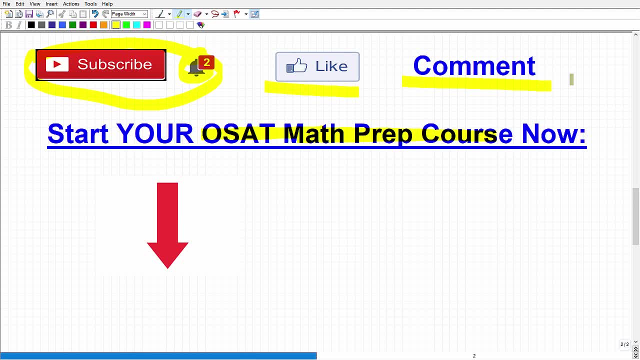 But, generally speaking, unless you've actually been in a classroom teacher and dealt with the pressures of you know responsibilities, of you know educating real live students in a classroom, And even though during this time there's a lot of remote learning going on, you know it's a, it's a, it's an important role that you play in our society.